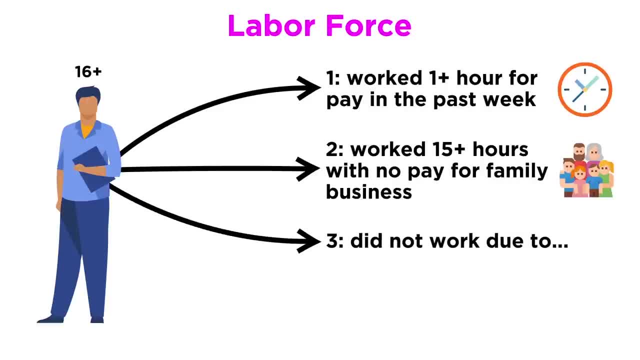 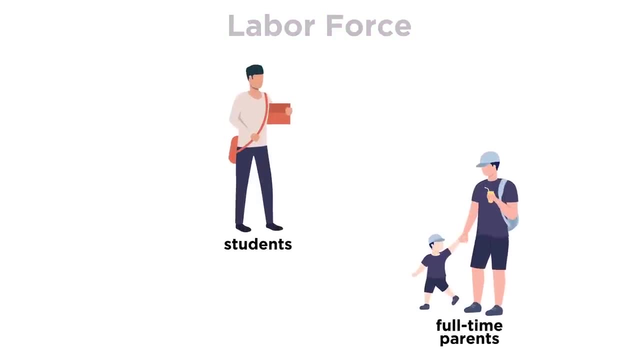 without pay in a family business Or three. they held jobs but did not work due to either sickness, vacation, labor disputes or bad weather. Typically, those who are not included in the labor force include full-time students, stay-at-home parents, retired people, active. 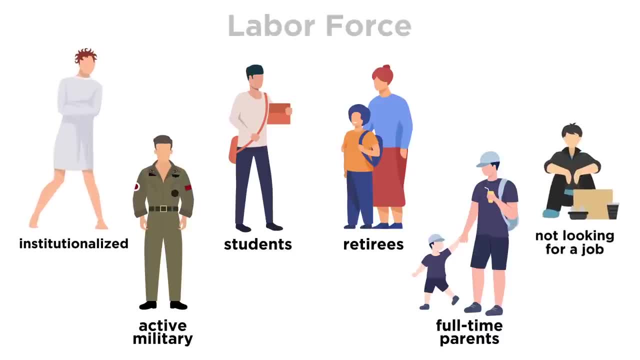 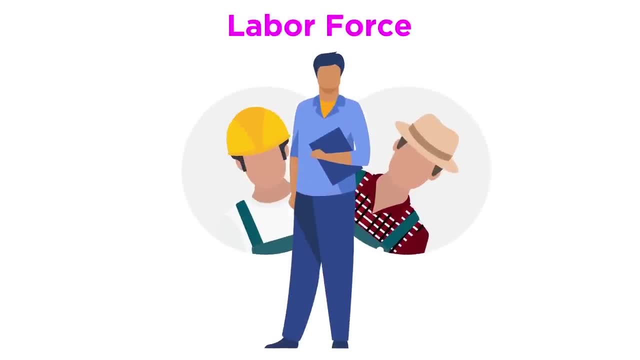 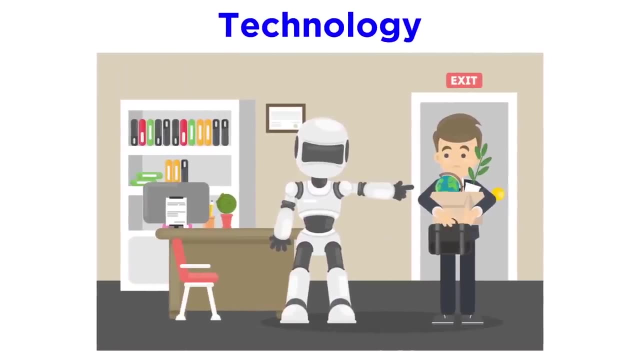 military, the institutionalized and the unemployed, And those who have given up looking for employment for an extended period of time. What if someone has more than one job? They're still only counted once in the labor force. Technology is constantly changing the labor force. In the early days of the United States, 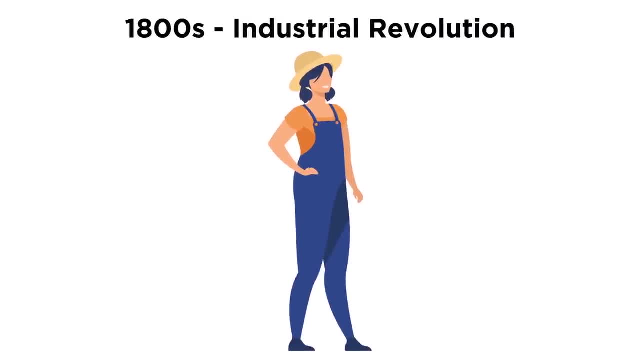 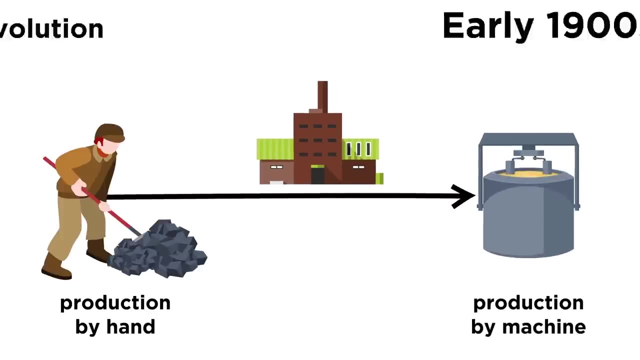 most citizens were farmers. Throughout the 1800s, however, the economy transformed due to the Industrial Revolution, a time of rapid economic expansion caused by the shift from agriculture and production by hand to factories and production using machines. By the early 1900s, heavy manufacturing had become the main driver of the American economy. 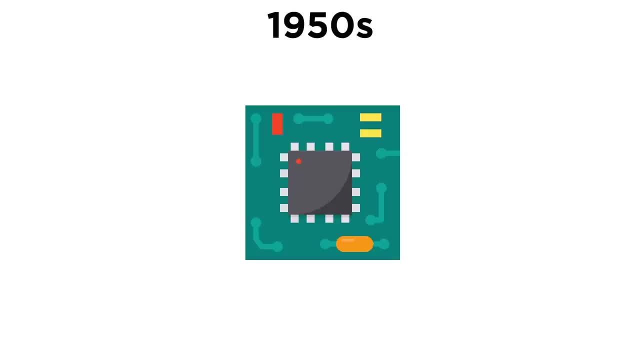 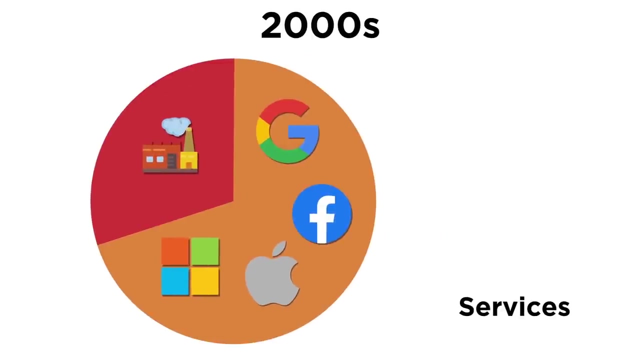 In the second half of the 1900s, a boom in electronics created a new wave of factory jobs. Beginning in the 1970s, the revolution in personal computers led to yet another boom Due to rapidly changing technology over the past few decades. service-producing: 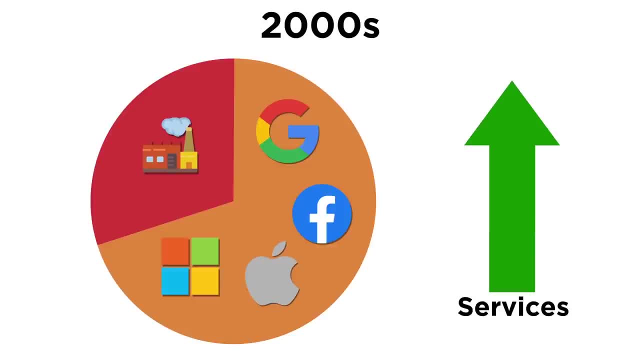 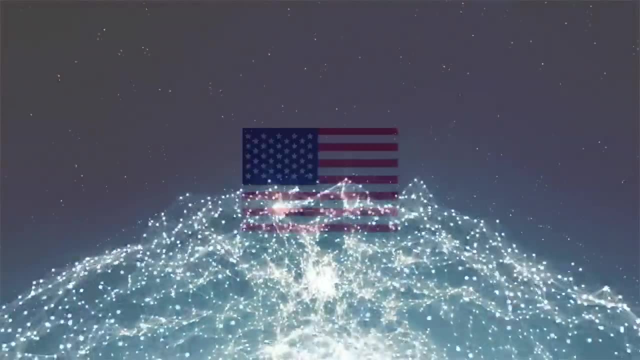 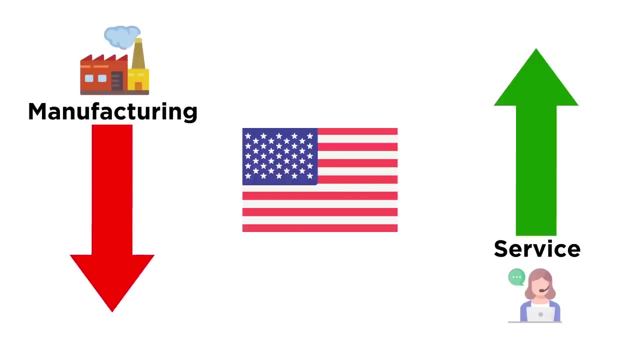 industries have been far outpacing good-producing industries. Globalization has also dramatically changed the labor force in recent years. While the number of service jobs has increased, the United States has lost millions of manufacturing jobs, mostly due to outsourcing and offshoring. 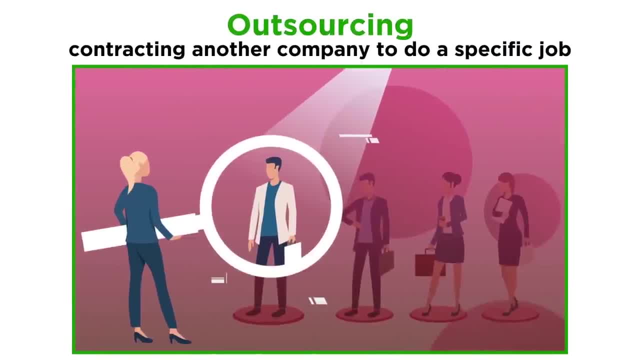 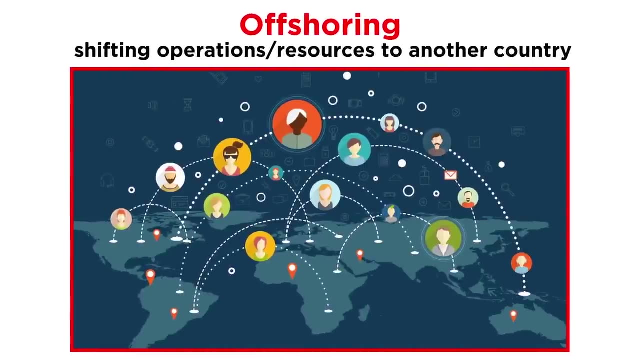 Outsourcing is when a company contracts with another company to do a specific job that would otherwise be done by a company's own workers. Most companies outsource work in at least some way. Offshoring is when a company shifts some of its operations or resources of production. 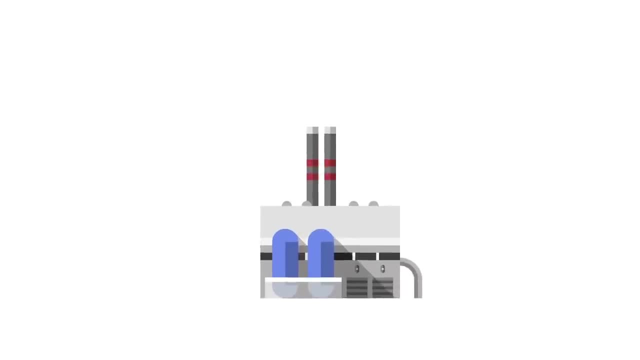 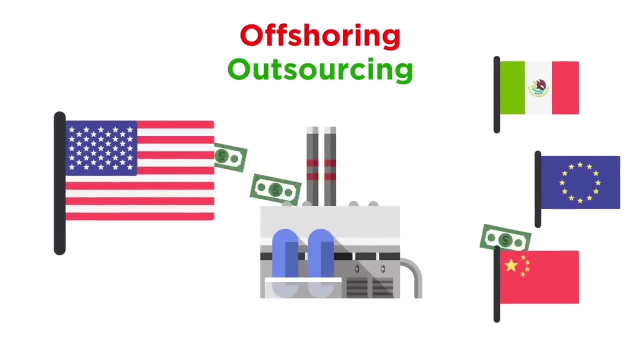 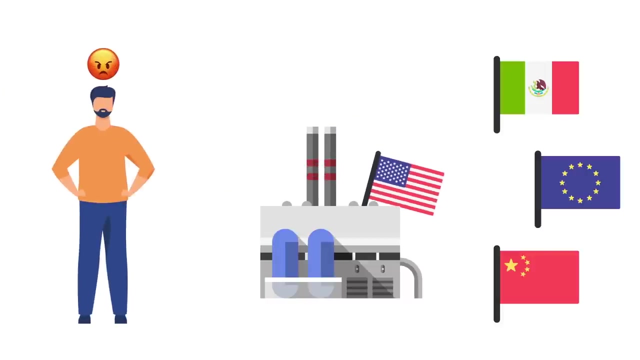 to another country. More often than not, companies outsource and offshore in order to save money, as they can pay workers in other countries less than workers in their own country. As less skilled manufacturing jobs moved overseas, the Americans who had filled these jobs had to